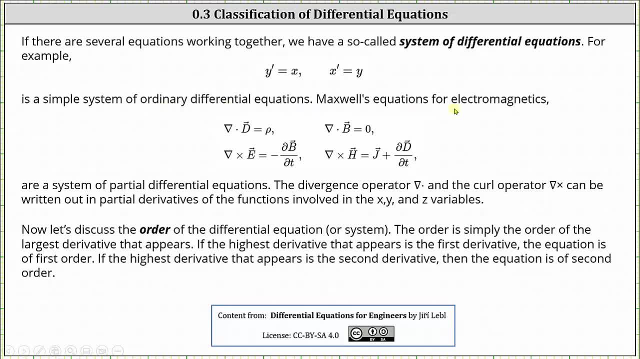 of ordinary differential equations. Maxwell's equations for electromagnetics shown below are a system of partial differential equations Recall from Calc 3,. the divergence operator and the curl operator can be written out in partial derivatives of functions involved in the X, Y and Z variables. 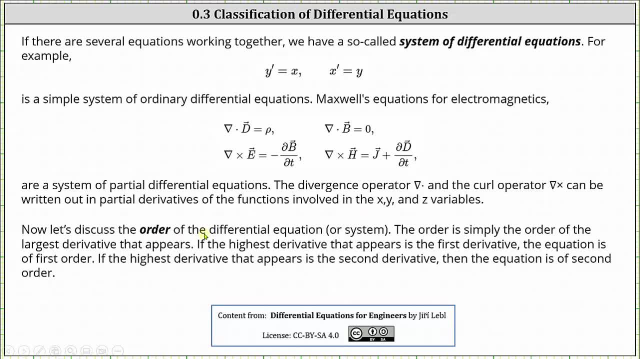 And now let's discuss the order of the differential equation or system. The order is simply the order of the largest derivative that appears. If the highest derivative that appears is the first derivative, the equation is of first order. If the highest derivative that appears. 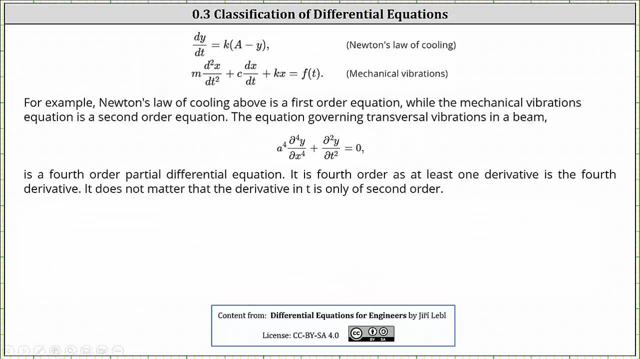 is the second derivative, then the equation is of second order. For example, Newton's law of cooling above is of first order because it only involves the first derivative, while the mechanical vibrations equation is a second order equation because the highest derivative is the second derivative. 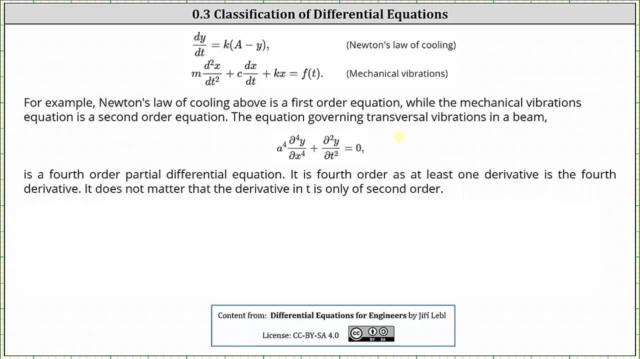 The equation governing the transversal vibration in a beam shown below is a fourth order partial differential equation. It is fourth order as at least one derivative is the fourth partial derivative. It does not matter that the derivative with respect to t is only of second order. 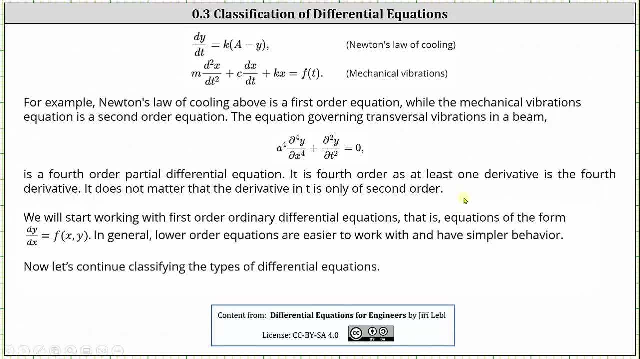 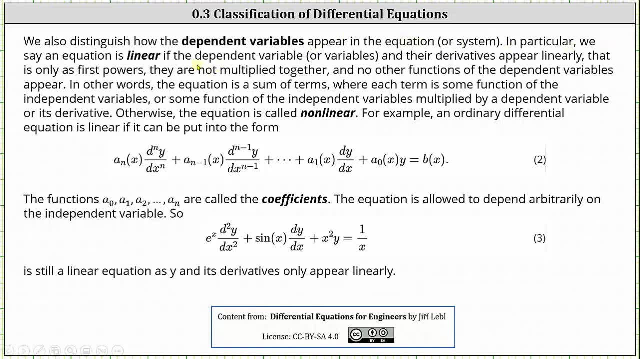 The equation is still classified as fourth order. We also distinguish how dependent variables appear in the equation or system. In particular we say, an equation is linear if the dependent variable or variables and their derivatives appear linearly. That is only as first powers. 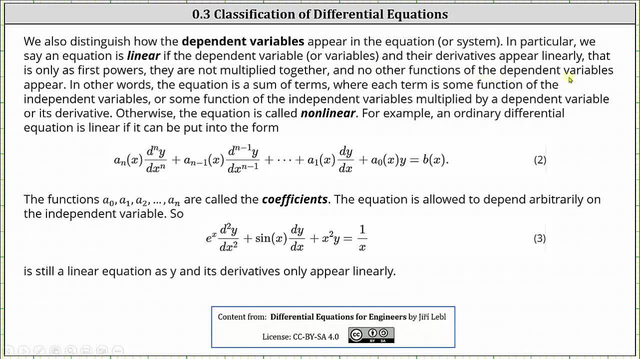 They're not multiplied together and no other functions of the dependent variables appear. In other words, the equation is the sum of terms, where each term is some function of the independent variables or some function of the independent variables multiplied by a dependent variable or its derivative. 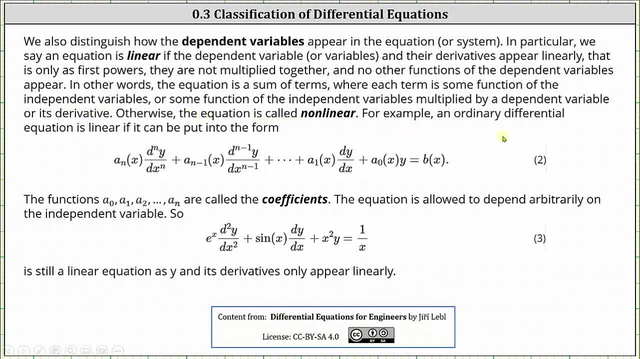 Otherwise the equation is called nonlinear. For example, an ordinary differential equation is linear if it can be written in the form shown below Notice. the equation is the sum of terms, where each term is some function of the independent variable x or some function of x multiplied. 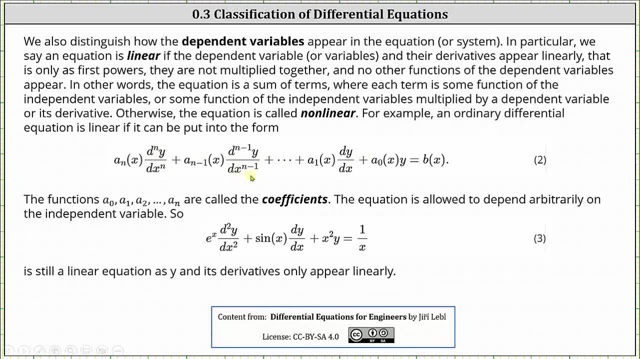 by the dependent variable y or its derivative. You may want to pause the video and study this form. The functions a sub zero through a sub n are called the coefficients, and the equation is allowed to depend arbitrarily on the independent variable. So the differential equation shown below, equation three: 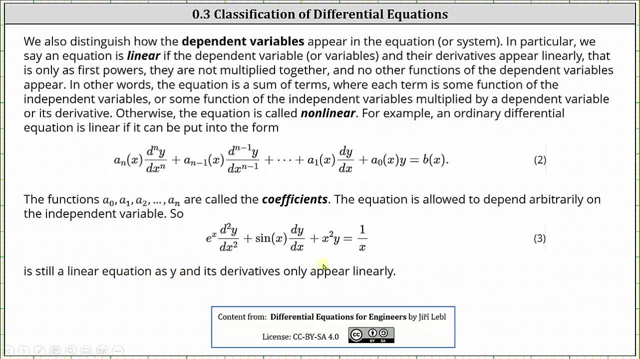 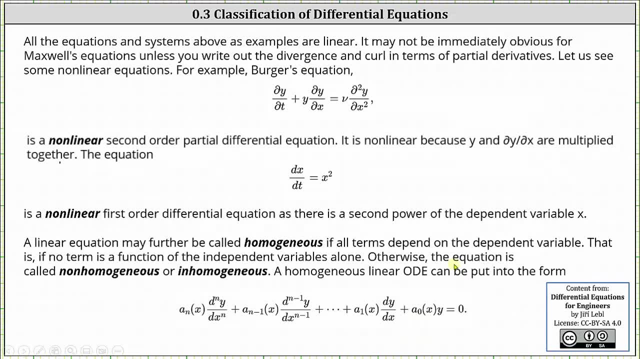 is still a linear equation as y and its derivatives only appear linearly, meaning raised to the first power. All the equations and systems above as examples are linear. It may not be immediately obvious for Maxwell's equations unless we write out the divergence and curl. 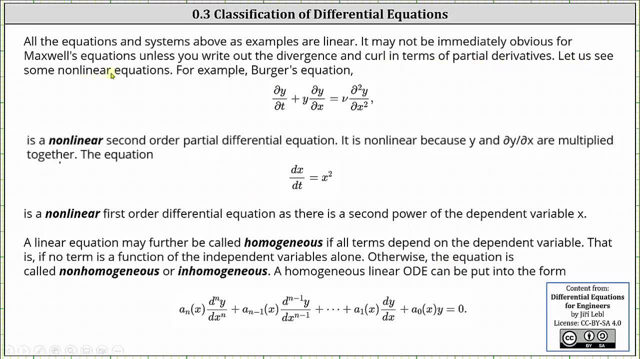 in terms of partial derivatives. Let's see some nonlinear equations. For example, Berger's equation shown below is a nonlinear, second-order partial differential equation. It is nonlinear because y and the partial y with respect to x are being multiplied together. The equation dx- dt equals x squared. 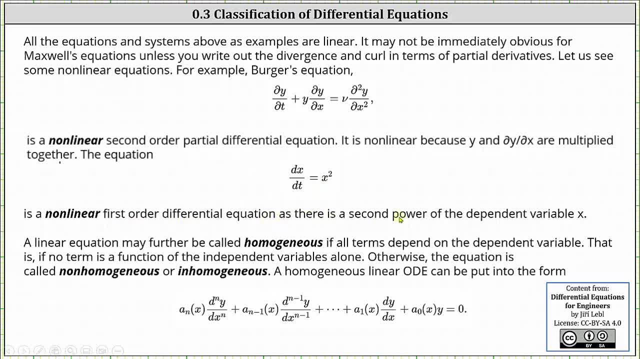 is a nonlinear first-order differential equation as there is a second power of the dependent variable, x. Because we have dx, dt in the equation. we know x is the dependent variable and t is a dependent variable. So because of the x squared, we have a nonlinear first order differential equation. 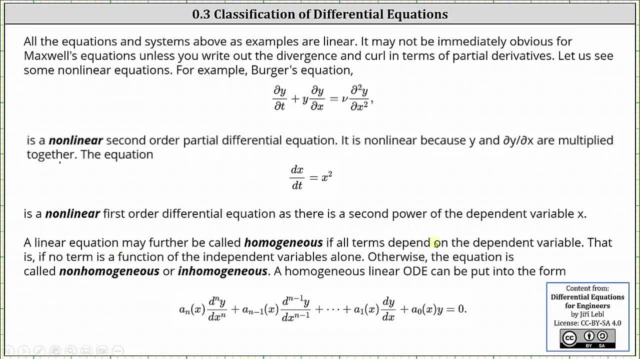 A linear equation may further be called homogeneous if all terms depend on the dependent variable, That is, if no term is a function of the independent variables alone. Otherwise, the equation is called nonhomogeneous or nonhomogeneous, or inhomogeneous or inhomogeneous. 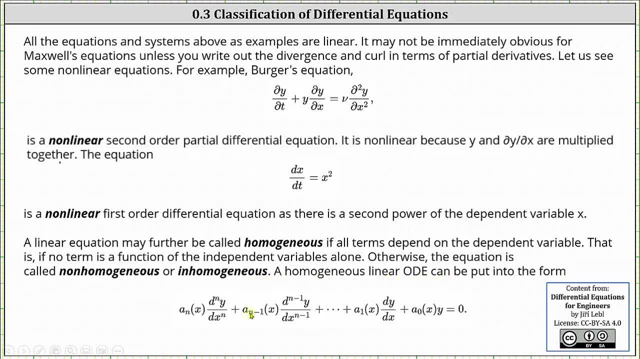 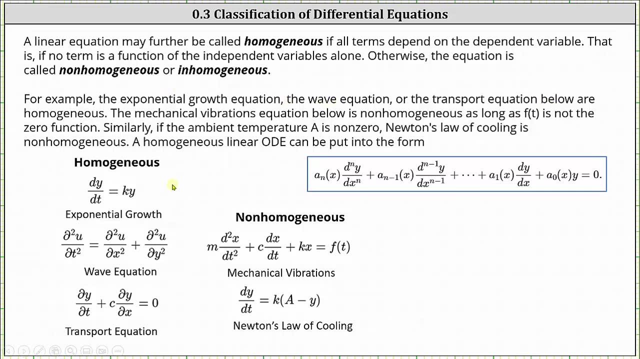 A homogeneous linear ODE can be written in the form shown below. Notice: no term is a function of the independent variable alone. For some examples, the exponential growth equation, wave equation and transport equation- all shown below on the left, are homogeneous. 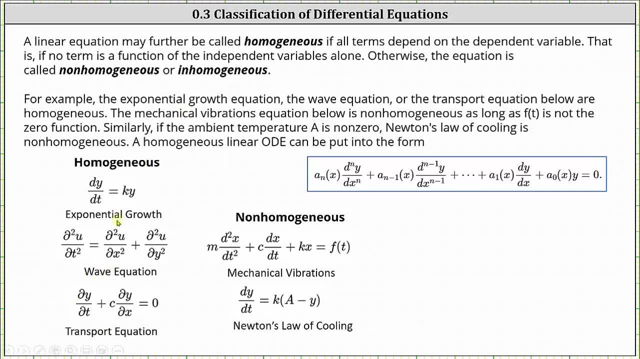 Again, no term is a function of the independent variable or variables. You may notice, for the first two equations the right side of the equation is not equal to zero, but that doesn't matter As long as we have a linear equation where no term is a function. 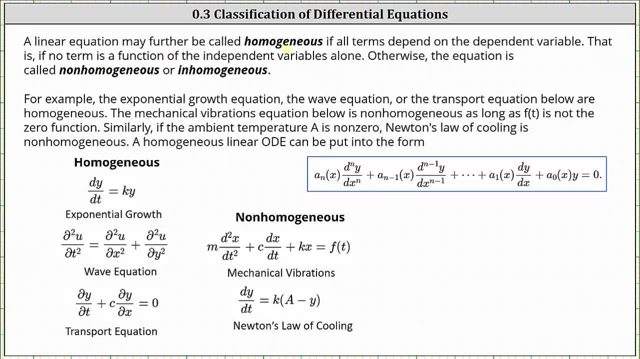 of the independent variables alone, we do have a homogeneous linear ODE. In contrast, the mechanical vibrations equation below is nonhomogeneous as long as f of t is not the zero function. Notice here: t is the independent variable. Similarly, if the ambient temperature A is nonzero, 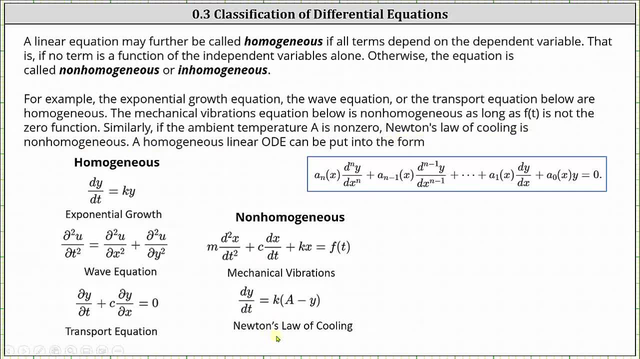 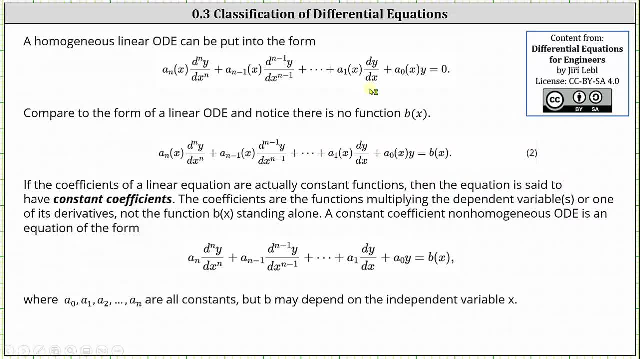 Newton's law of cooling is also nonhomogeneous. Again, a homogeneous linear ODE can always be written in the form shown here in the blue box. If we compare the form of a homogeneous linear ODE to the form of a linear ODE, 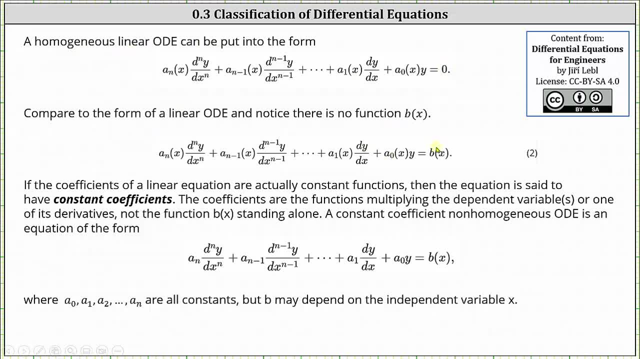 notice: for the homogeneous linear ODE there is no function b of x. If the coefficients of a linear equation are actually constant functions, then the equation is said to have constant coefficients. The coefficients are the functions multiplying the dependent variable or one of its derivatives, not the function. 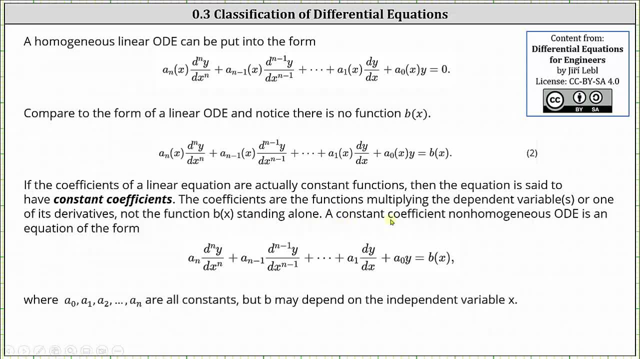 So if we compare the functions of a linear equation with a nonhomogeneous linear ODE, we can see that the function b of x is not the function b of x standing alone. A constant coefficient- nonhomogeneous ODE is an equation in the form shown below. 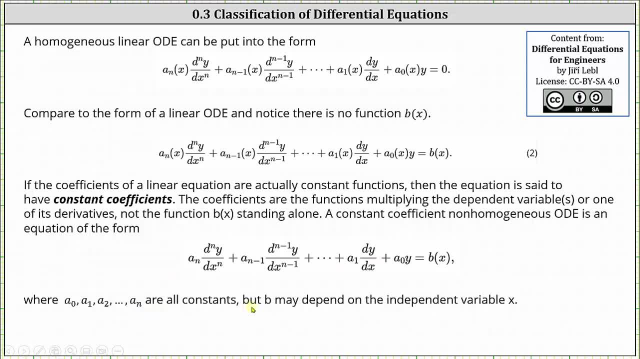 where a sub zero through a sub n are all constants, but the function b may depend on the independent variable x, which is shown here on the right. For some examples, the mechanical vibrations equation below is a constant coefficient, nonhomogeneous second order. 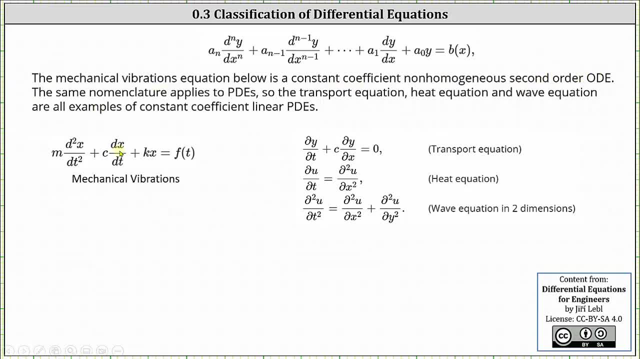 nonhomogeneous. second order differential equation: The same nomenclature applies to PDEs. So the transport equation, heat equation and wave equation, all shown below, are examples of constant coefficient, linear, partial differential equations. And then, finally, an equation or system is called autonomous. 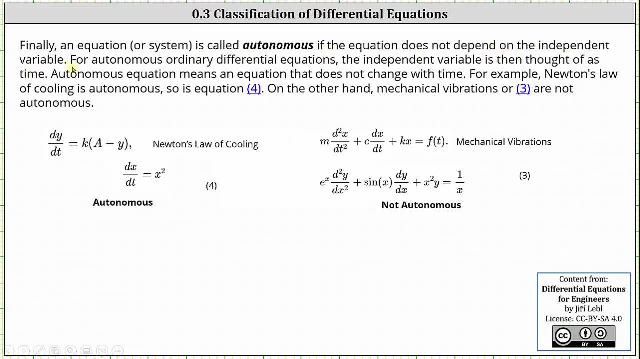 if the equation does not depend on the independent variable. For autonomous ordinary differential equations, the independent variable is then thought of as time. Autonomous equation means an equation does not change with time. For example, a Newton's law of cooling, again shown below, is autonomous. 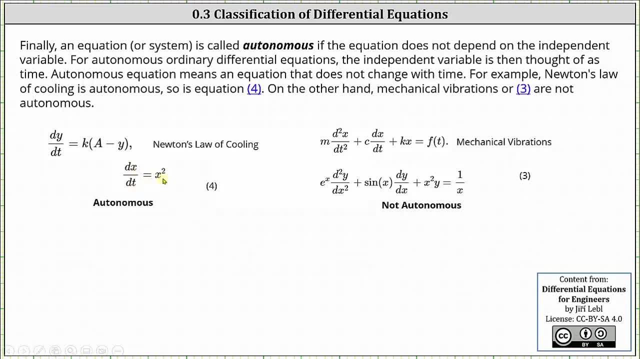 and so is equation four. the equation dx dt equals x squared. Notice: both equations do not depend on the independent variable t. On the other hand, the mechanical vibrations equation and equation three below are not autonomous. The mechanical vibrations equation is not autonomous. 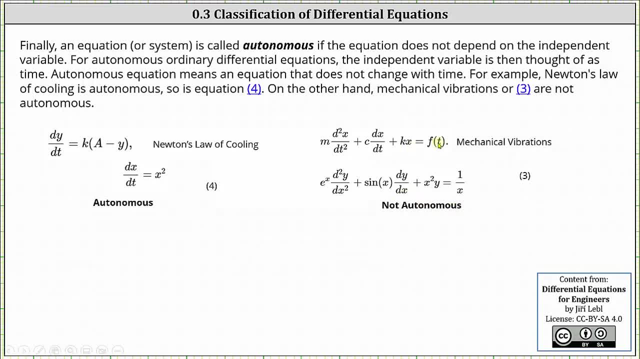 because it does depend on the independent variable t, and equation three is also not autonomous because it depends on the dependent variable x. I hope you found this helpful.